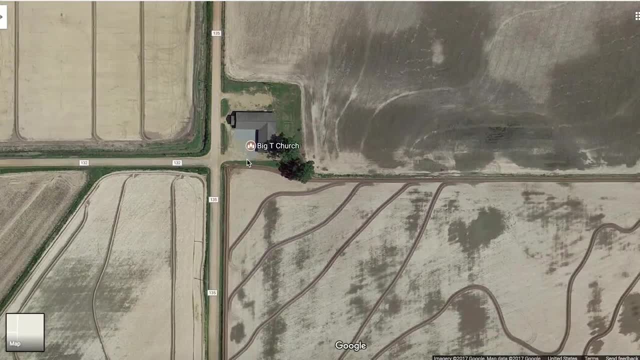 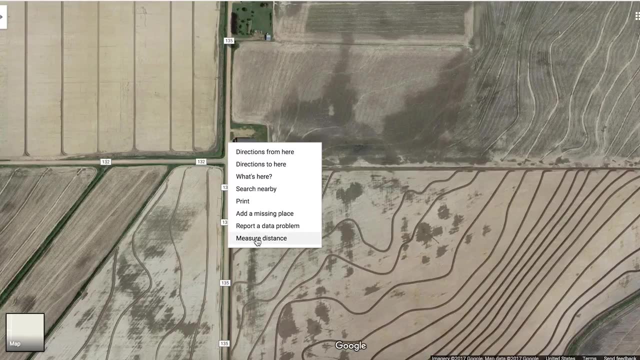 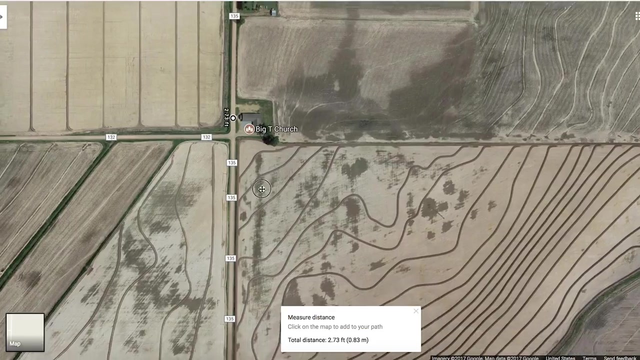 the church is down the road. I'm going to show you exactly here. If we will right-click, you can see where there is a button that says Measure Distance. You click on the Measure Distance Now. you click on the map. Now we're going to drag down all the way down. 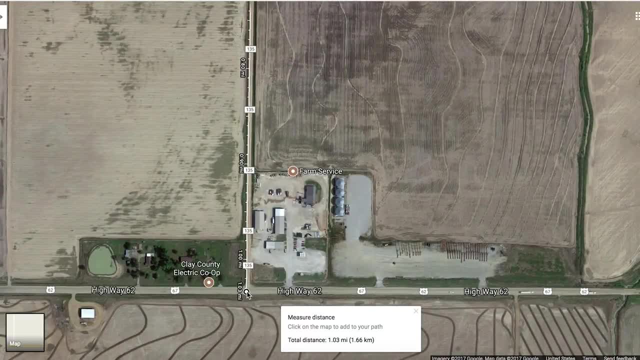 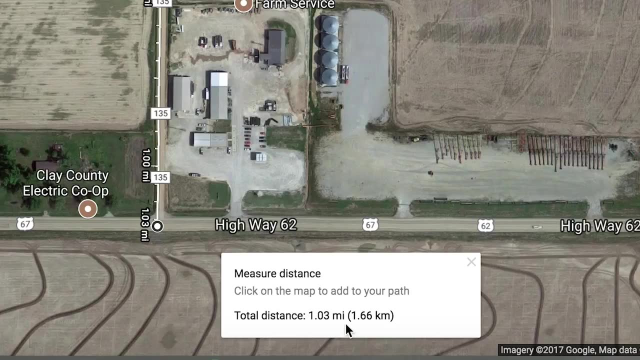 here to the highway and we will click there. Let's see on the bottom of your screen. Check this out. Total distance: 1.03 miles. So there you have it. You can see exactly how far something is, but don't click off the. 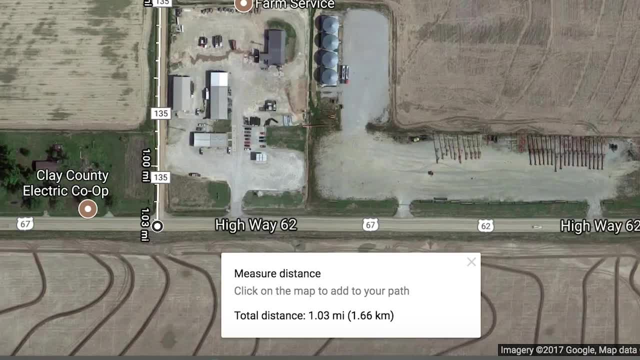 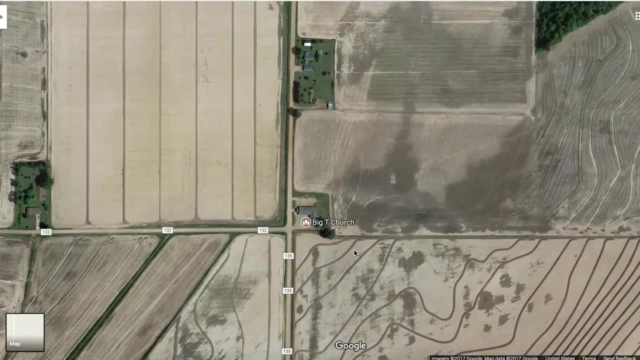 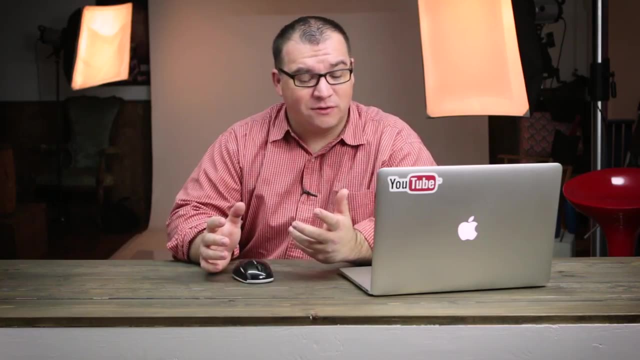 video, because it gets even more interesting than that. Let's right-click and clear Measurement. We're going to go back up here to the church building. Zoom in as close as we can now. This could be useful for contracting. This could be for contractors or someone that's wanting to get kind of a rough estimate. 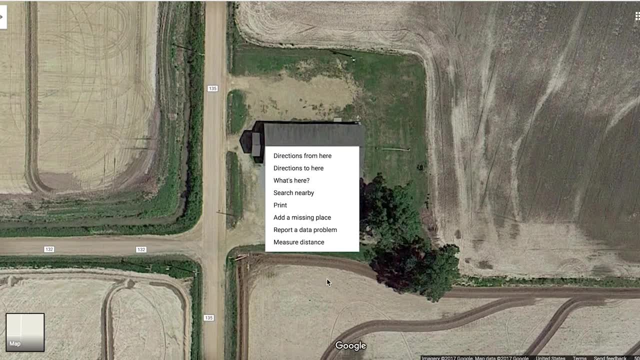 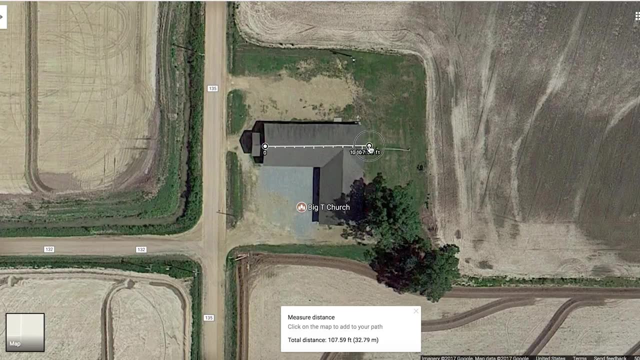 on something. We can actually right-click on the top of this roof Measure Distance and then we can click on the very back side of it. You can move these in and out to get them pretty close. See where the zero is. Drag that out here. You can look at that now. 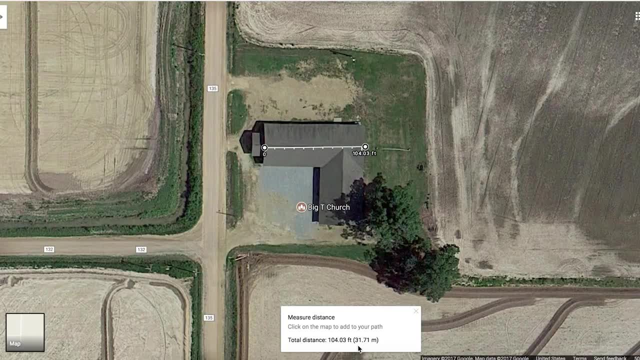 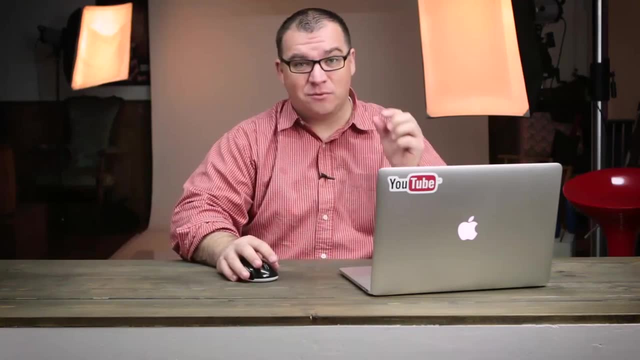 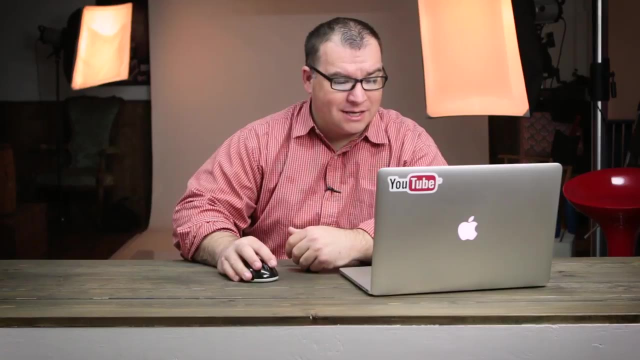 and you can see that the roof is going to be a little bit more enough. You're going to have to roof length right there is like 104.03 feet. Now you and me both know that from this distance we're not going to get it down to the exact inch. That's as far as we can zoom in. but you realize. 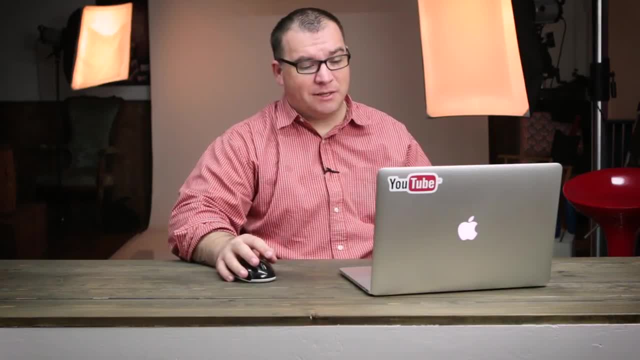 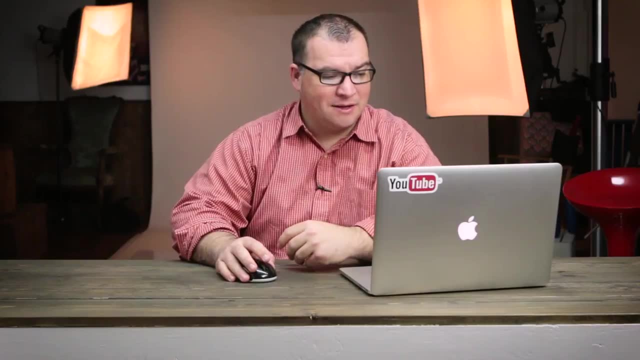 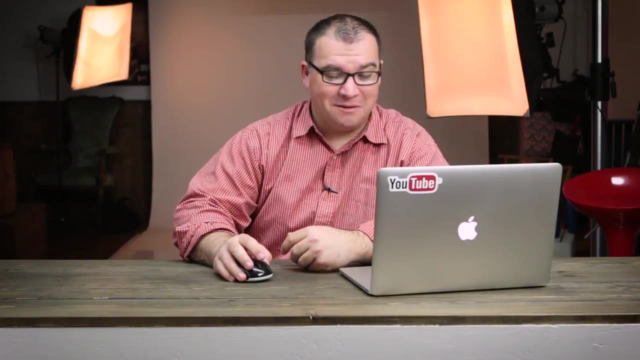 that would get somebody a fairly close estimate if you needed to know something. This tool, I think, could be useful for several different things. I actually measured the length of our football field, just to kind of check it and see how it was. I measured my father's house. 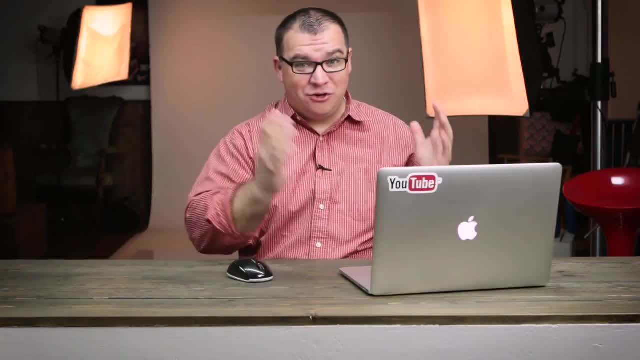 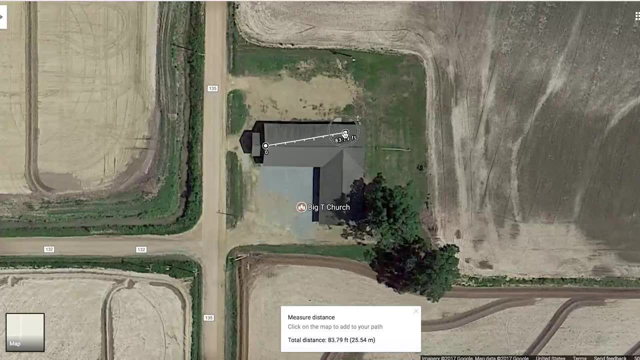 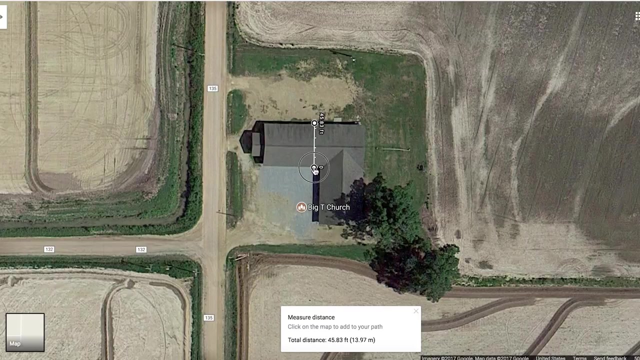 to get an idea of that. There's many things I think that you could use this measurement tool, for It's kind of endless. You can measure small things. You can move this down if you want to to measure the width, You can look here and we will measure the width of the church here. 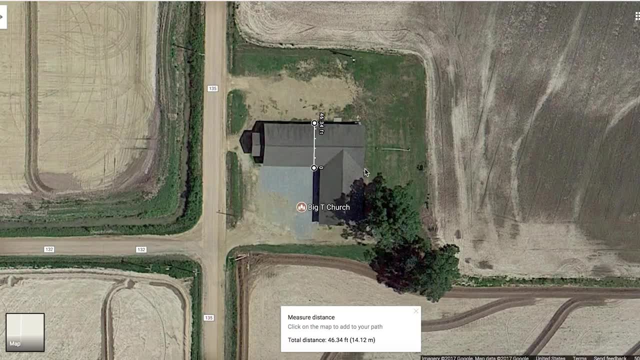 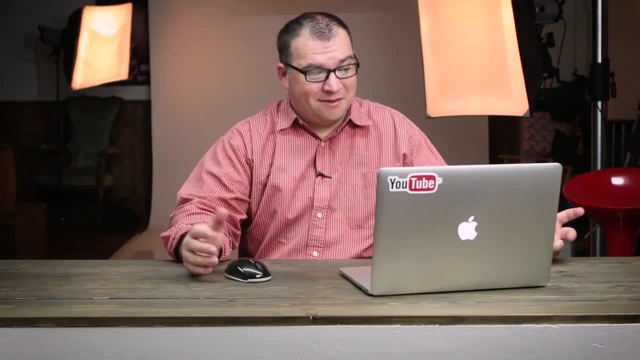 It looks like measuring that roof from there is 46 feet. I know the inside of our church building is 40 foot wide. So yeah, that gives you an idea of kind of how this works. I think it's pretty cool. Let me show you another. 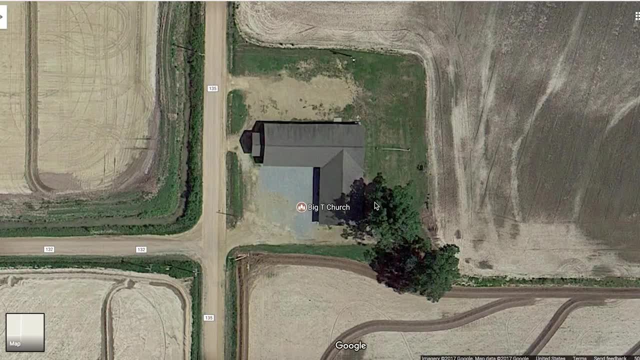 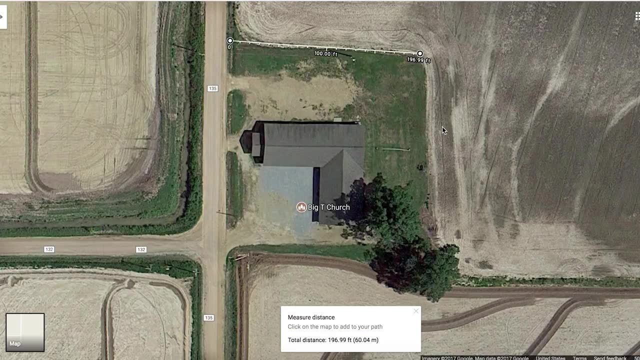 cool thing. Let's clear this measurement here Now. if I wanted to outline our church property to kind of see what kind of distance we have, I can right-click, I can measure, I can click over here. Now you can connect these. You don't have to draw just one line. So we're going to connect. 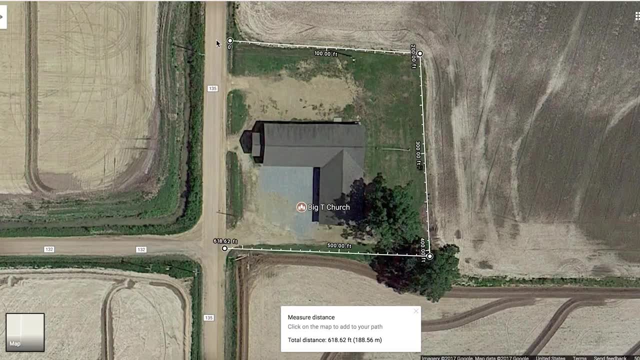 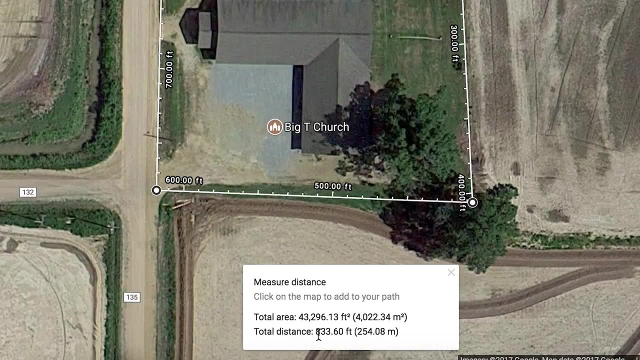 this somewhere Over here, Go back here and then finalize it Now. look at the distance. Now it'll tell you the total distance around the perimeter would be 833.6 feet, but it gives you a total area. So there's 43,296.13 square feet in this property. I think that's very useful. 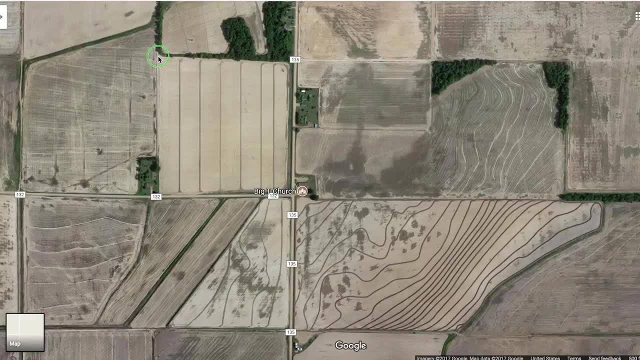 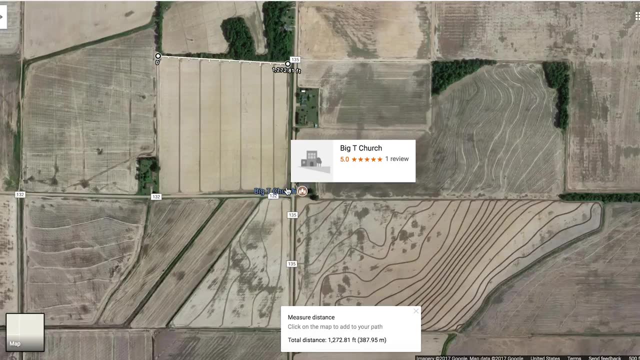 This could be used in agriculture or whatever. If you're looking at this map, we will check this field out here, this right across from the church. We will measure it out as well. Click the marks and let's see if we can get this to work. That gives us a rough. 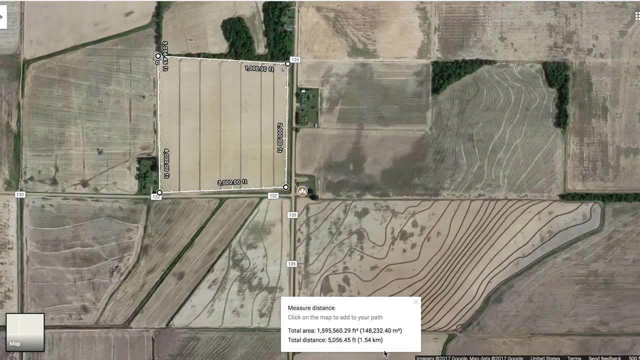 estimate. there It looks like 1.5 million square feet. So yeah, I guess you could figure that out to kind of know how many acres that would be. I think this is useful. It's a quick tip, something that I didn't know that. 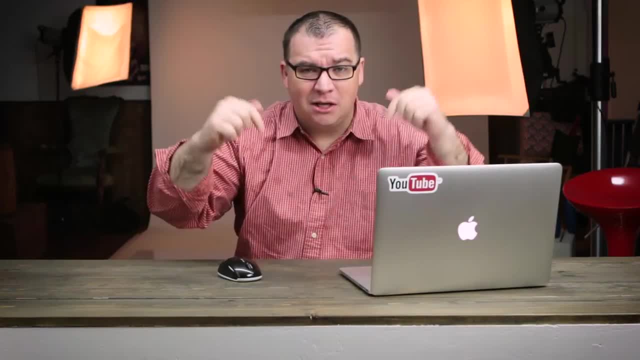 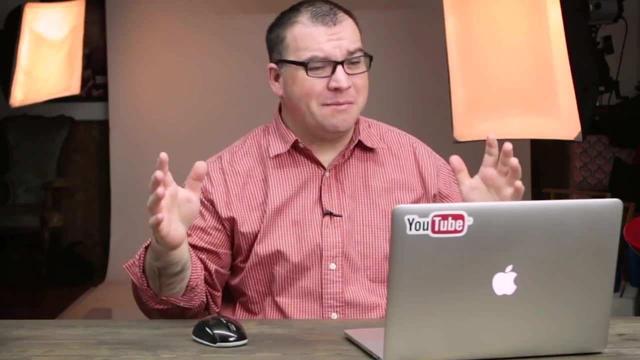 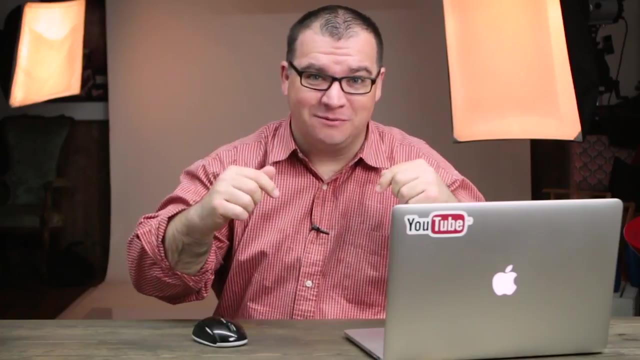 maybe you already knew. Leave me a comment down below. Let me know: is this something that you knew existed, or is this new to you as well? Also, let me know what kind of idea that you have that you could use this measurement tool for. I'd like to hear that down in the comments below, I hope. 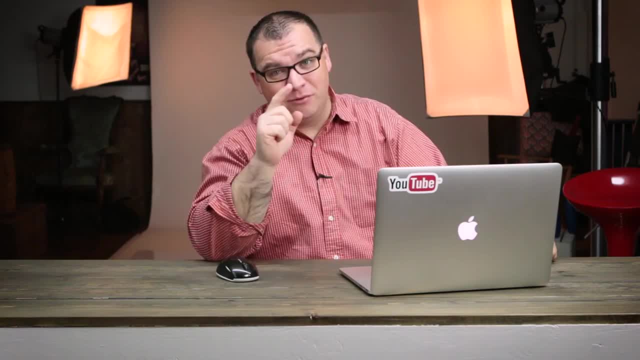 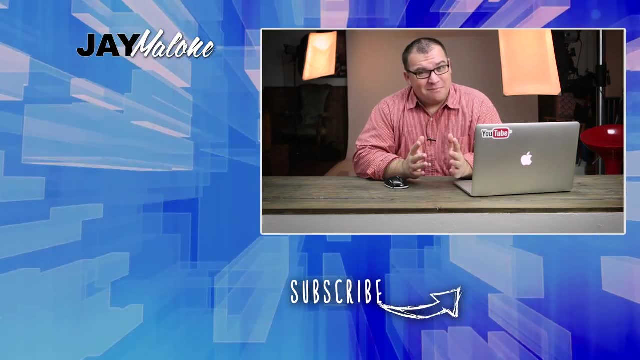 you enjoyed this video. If you did give it a big thumbs up, That would let me know that you liked this video, And if you want to see some more of my videos, click over here. And if, for some reason, you're not already subscribed to this channel, 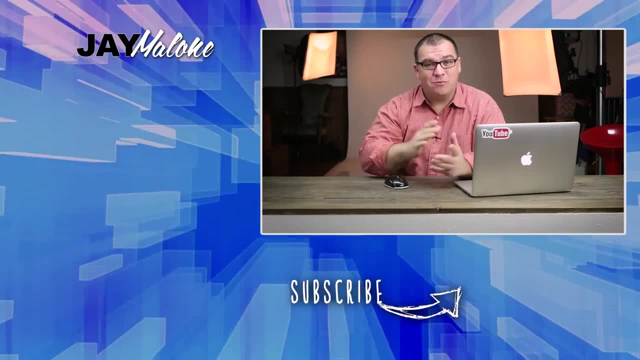 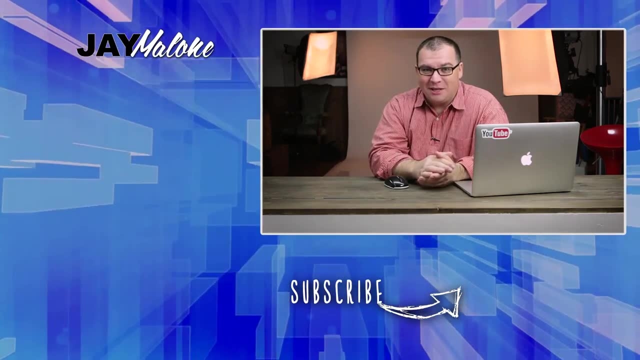 then click my face in the circle icon down below this video. That will get you subscribed. Thanks for liking, commenting and subscribing And until next time, God bless.